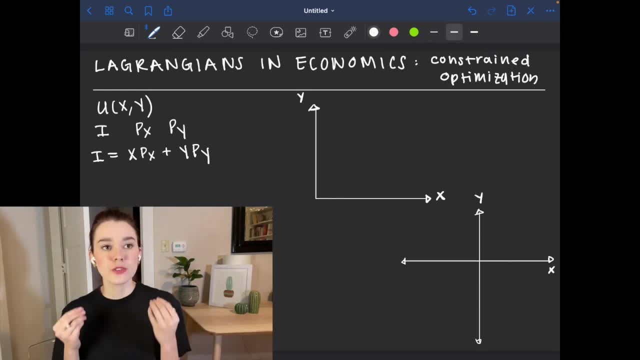 That should be review. And what did we do with this? Well, we want to pick the best combination of x and y that makes us the happiest. We want to maximize our happiness or our utility level. but we can't just blatantly maximize our happiness because, also, we only have so much money. We have a constraint. 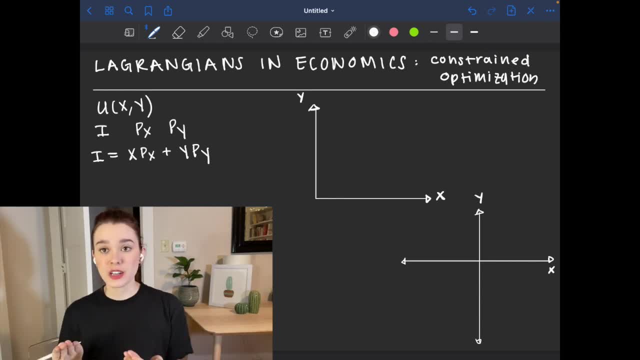 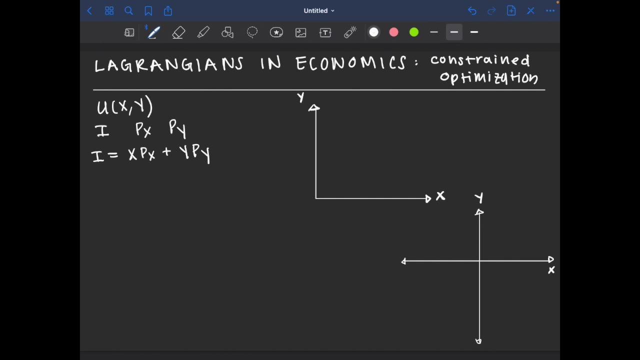 which is our budget constraint And so constrained optimization, which is what we use the Lagrangian method for, is just a way to maximize my utility with respect to my budget. Before we get into the actual Lagrangian method, let's remind ourselves that we have indifference curves. 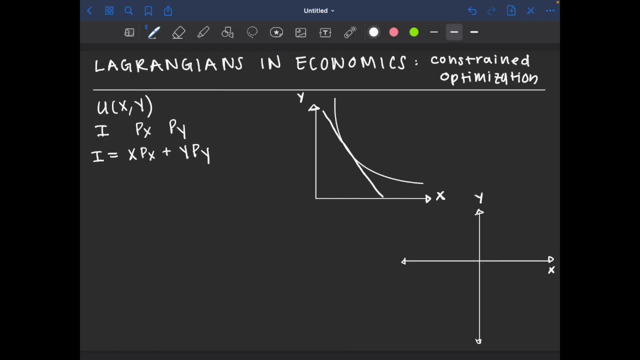 and also that in our econ 101 classes we saw that the optimal bundle was always this tangency point, when the indifference curve was just touching the budget constraint, And we said that this point we could find it when the slopes of the indifference curve and the slope of the budget constraint were equal. 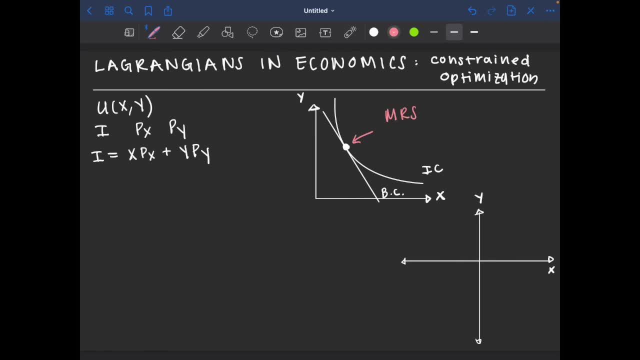 They're the same. So the slope of my indifference curve is equal to the negative marginal rate of substitution And the slope of my budget constraint is equal to the negative ratio of the prices. Since there's a negative on both sides, I can just get rid of that and ignore it. 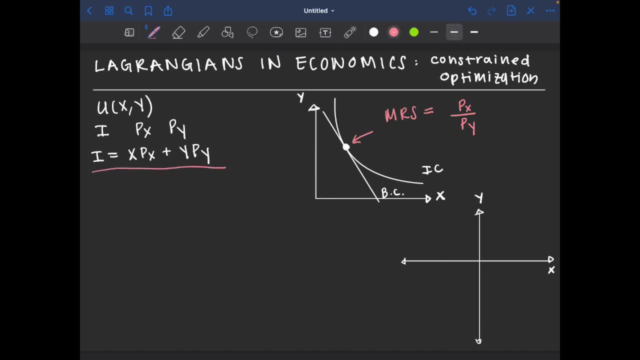 And we would use this and our budget constraint, We would combine those in order to find the optimal bundle. Well, that's always our goal: to find x star and y star, We said. given our budget, given prices, this combination of x and y will make me the happiest. 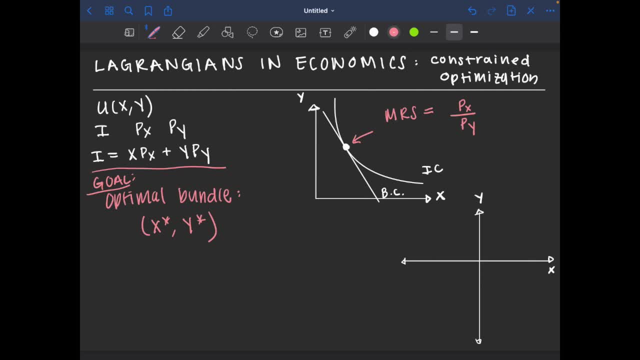 So this was our goal And we did this in Econ 101.. Now we're going to use the Lagrange method to find this, because sometimes we're using more complex formulas or more complex utility functions and we want- We want to be able to do it in a little bit more rigorous of a way. 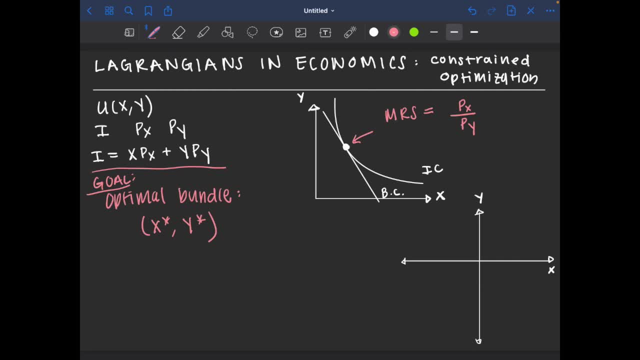 Before we get into the Lagrange method, let's review one more thing. that is from Calc 1.. In Calc 1, you might have been asked to find where the maximum point of a function was. So what if we have f of x equals negative x squared? 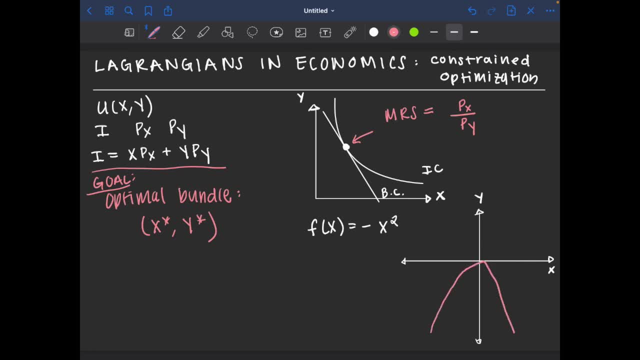 On my graph that looks kind of like this And I can look at my graph and see that the maximum point is right. But how would I find that mathematically? I would take the derivative of my function and set that equal to 0.. 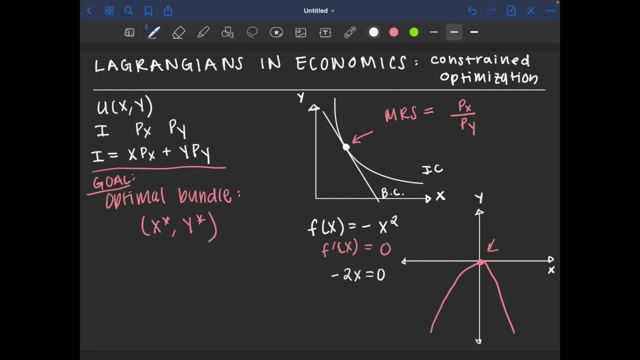 So if I do that really quick, I would get minus 2x equals 0.. If I solve for x, it gives me x star equal to 0. So that means that my maximum point happens at x star. I've maximized my function at x star equal to 0. 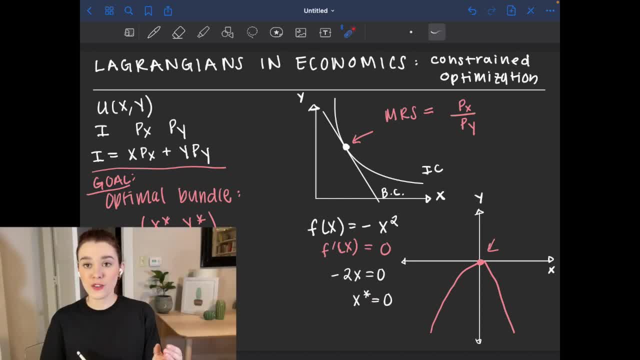 The Lagrange method is just. It's a fancier way of doing this optimization. In this Calc 1 example, we only had one input, We had x. Here we have x and y going into a function, And so we can no longer just take normal derivatives and set them equal to 0.. 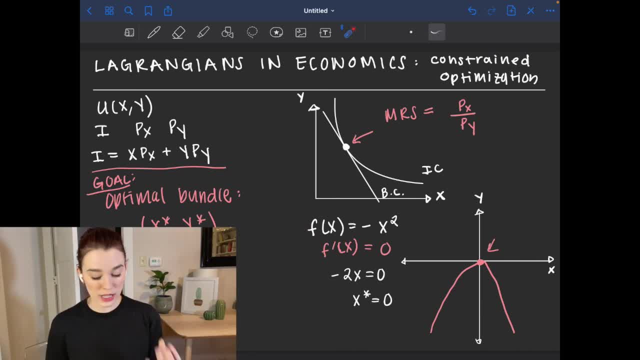 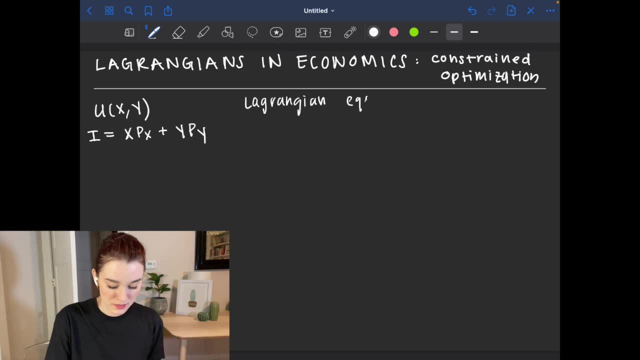 We have to use something more complex. So let's actually get into the Lagrangian. We start with the Lagrangian equation. So I start with this curly L. This is just to signal that This is a Lagrangian function or equation. 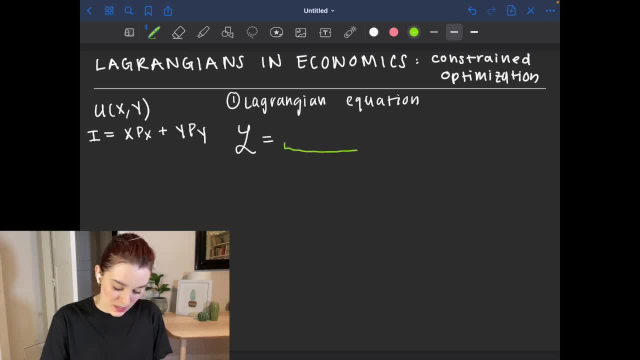 That's all. Then I am going to put in something called my objective function Plus lambda, which is called my Lagrangian multiplier, And I'm going to multiply that multiplier by a constraint. So this is the pattern, the general pattern of a Lagrangian. 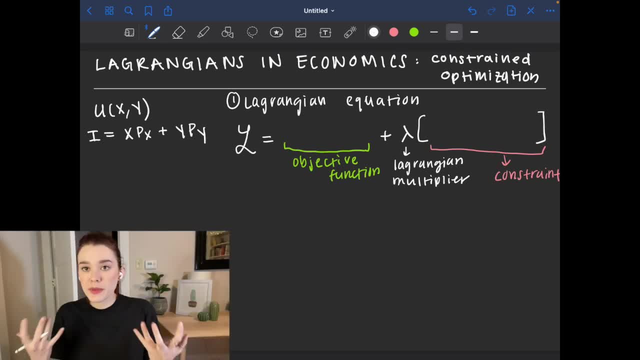 The objective function. that's my objective And what's my goal here. I want to maximize my utility. right, I'm trying to find the bundle x star and y star that maximizes my utility. So I would write my utility function. 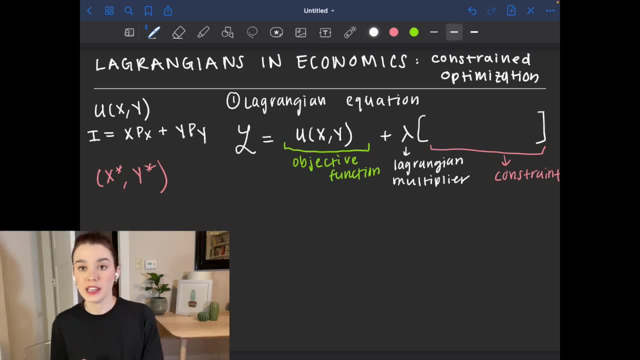 And I'm leaving everything in general here. I'll do an example in another video. The constraint is a little bit more simple to understand. what goes there, It is just the constraint. What's our constraint? It's the constraint, It's the constraint. 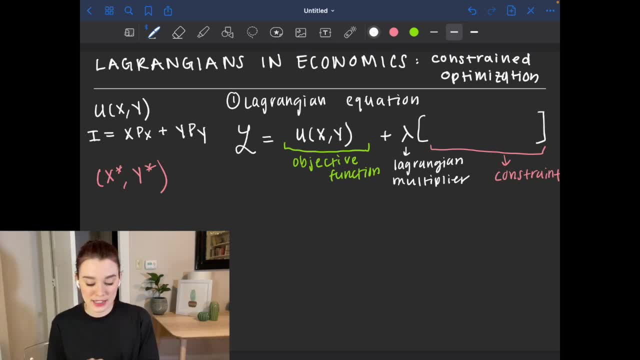 It's the constraint In this scenario, it's my budget constraint. But before I write that in there, I actually have to do one quick step to my budget constraint. So I need to rearrange it so that there's zero on one side of the equation. 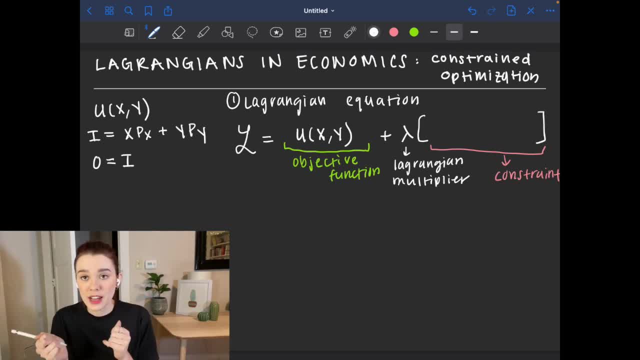 It doesn't matter what you put where, as long as your math is correct and zero is on one side. So for me, I'm going to subtract these two terms to the other side. Now I can write this part in my constraint box. 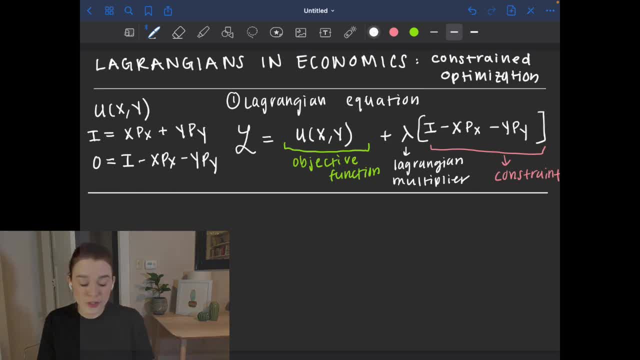 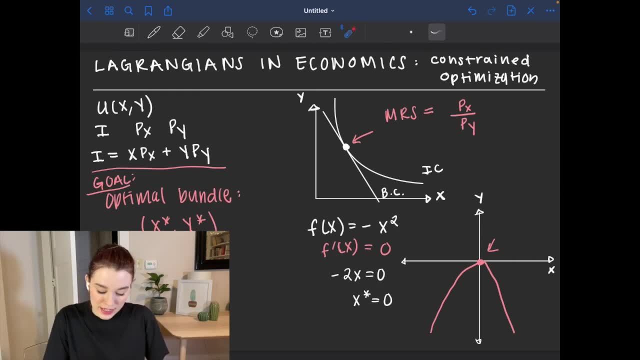 Now what I want to do is I'm going to take something called the first order conditions, which we call FOC. Let's go back to our Calc 1 example really quick. This right here is technically a first order condition. A first order condition is a derivative that I've set equal to zero. 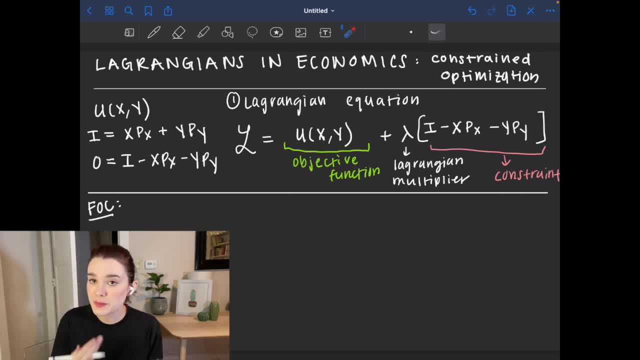 When we have multiple variables, multiple things to take derivatives with respect to, we have a whole set of them. We have multiple first order conditions. So I have three first order conditions. in this case, I have a first order condition with respect to x. 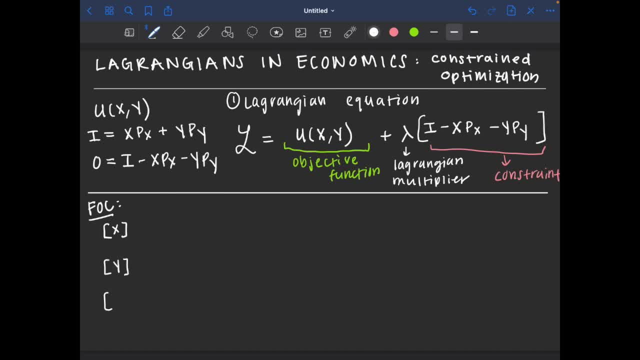 a first order condition with respect to y and a first order condition with respect to lambda, And all I'm going to do is take the derivative of the Lagrangian with respect to y and set that equal to zero, And I'll do that with respect to that variable. 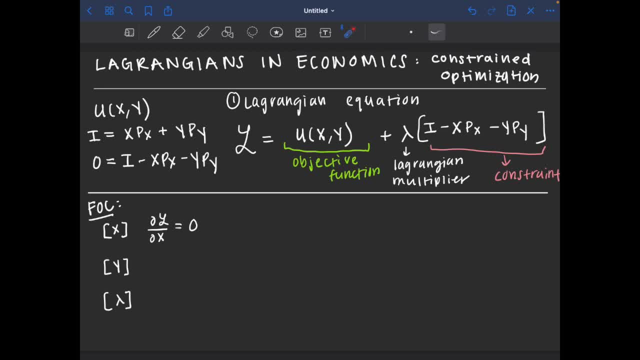 and set that equal to zero. In this case, not only do we have multiple variables, we also have a constraint, And so I need to take the partial derivative of the Lagrangian with respect to x, And I'll do that with respect to y. 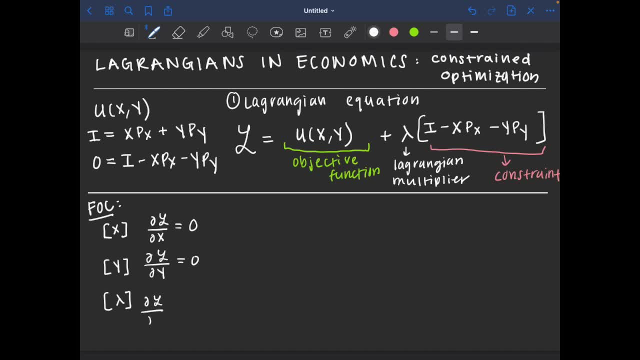 and set it equal to zero, And with respect to lambda, and set that equal to zero. I can take the partial derivative of the Lagrangian with respect to x by taking the partial derivative of the utility with respect to x. 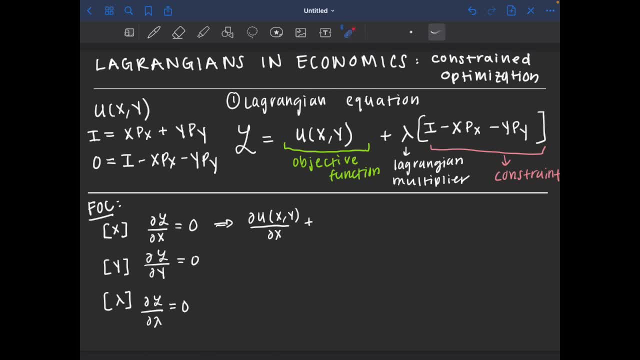 plus this one, I have a lambda out front that is multiplied by that, And I also have a minus px multiplied by x, And so then I set that equal to zero. I can do a similar thing here. The partial derivative of the utility function with respect to y. 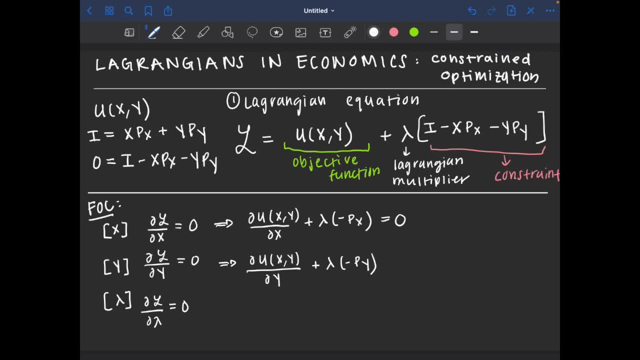 plus lambda, times minus py. So this time I've just taken the partial derivative with respect to y, set that equal to zero, And when I take the partial derivative of the Lagrangian with respect to lambda, I actually just get the budget constraint back out. 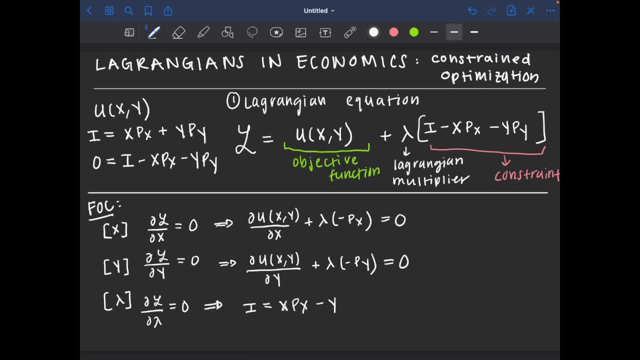 So when I'm solving these, I usually don't write this out Because I know it already: it's the budget constraint. What I do do is I make a mental note that my budget constraint technically will be one of my first order conditions. 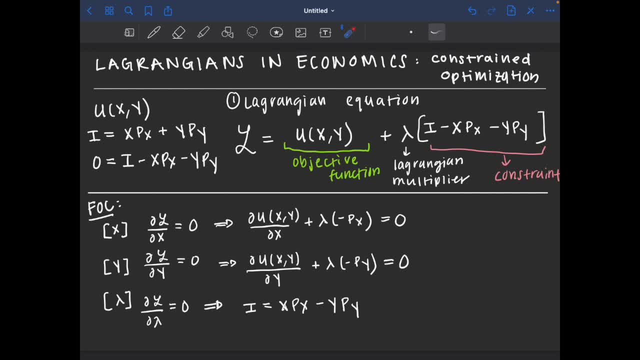 I also like to think of these as optimality conditions. These are kind of three conditions that my optimal bundle- x star and y star- is going to satisfy. So I can simplify these a little bit more and it will hopefully make sense why I'm doing that. 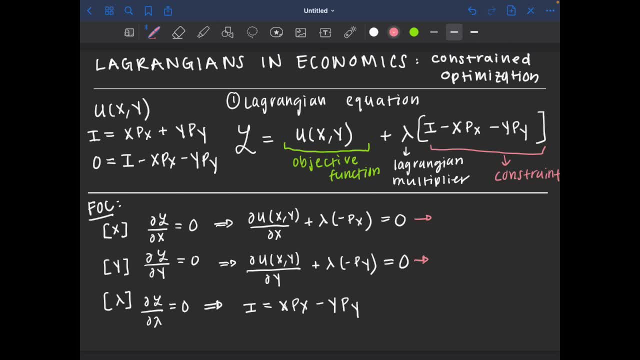 We'll draw a connection to what we learned in Econ 101.. So if I solve for lambda in both of these first two conditions, I would get lambda is equal to well instead of the partial derivative of utility with respect to x. 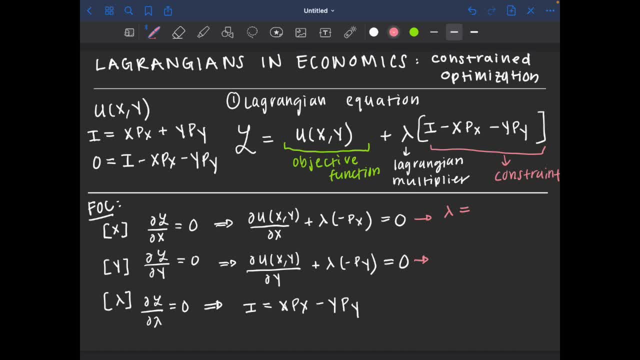 I can call that the marginal utility of x, And I've divided by the price of x. Here I would get the marginal utility of y. So this is equal to this And this is equal to this Over the price of y. 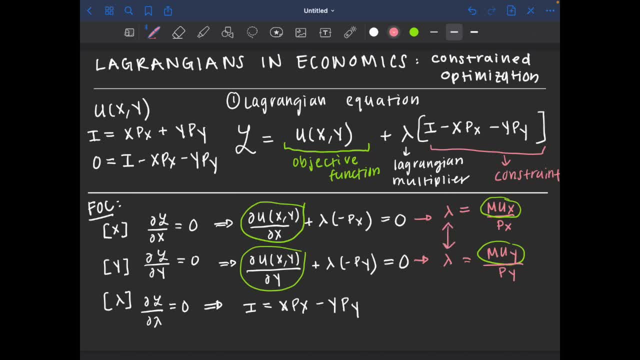 And finally, I could set those lambdas equal to each other- I like to think of lambda as a link- And that would give me the marginal utility of x over the price of x. equals the marginal utility of y over the price of y. 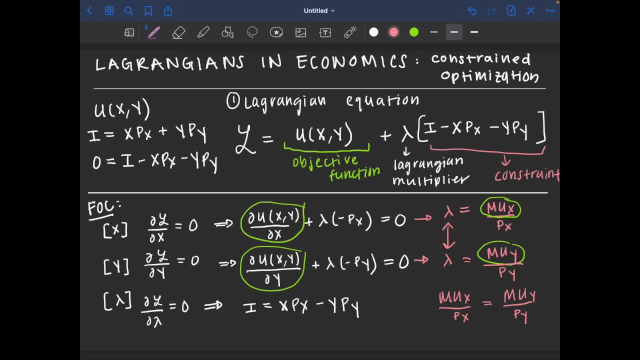 Well, if I simplify a little bit further, just one more step. I cross multiply, then I would get: the marginal utility of x over the marginal utility of y equals the price of x over the price of y. This seems awfully familiar.